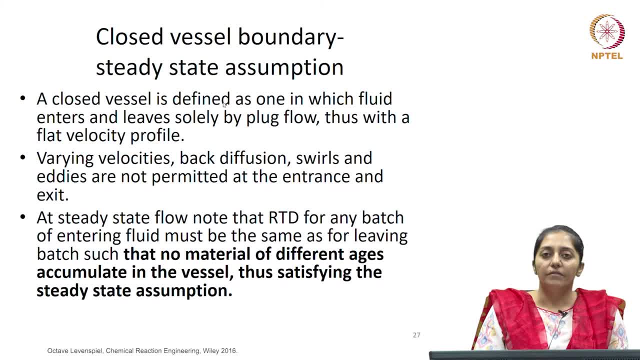 We spoke about the tracer experiments where different kinds of inputs can be given and at the exit the profile is noted how the tracer is coming out from the reactor with time. So we discussed specially the two types of inputs. one was the pulse input and the other 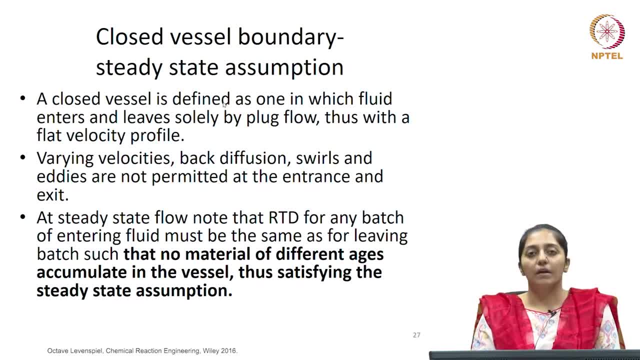 was a step input Then, where we came across the F curve and how E curve is related to F curve. Now we will talk about the steady state assumption or the closed vessel boundary. So a closed vessel is defined as one in which the fluid enters and then enters into the 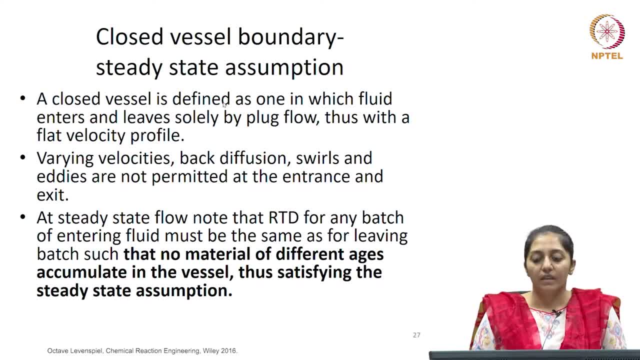 reactor and leaves solely by plug flow, Thus with a flat velocity profile, which means there is no velocity gradient. Now varying velocities or back diffusion, swirls and eddies. they are not permitted at the entrance or at the exit. Now at steady state, please note. 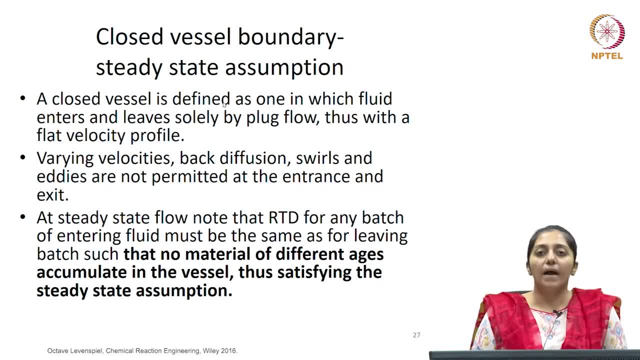 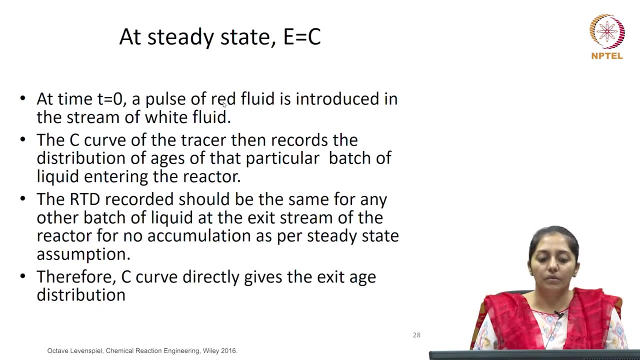 that the residence time distribution for any batch of entering fluid must be the same as for the leaving batch, such that no material of different ages get accumulated in the vessel, thus satisfying the steady state assumption. So at T is equals to 0 if a pulse of red fluid 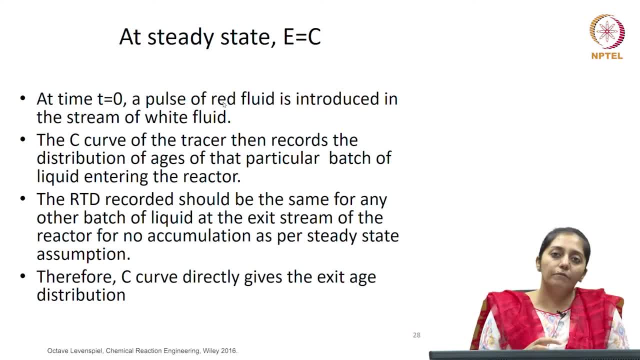 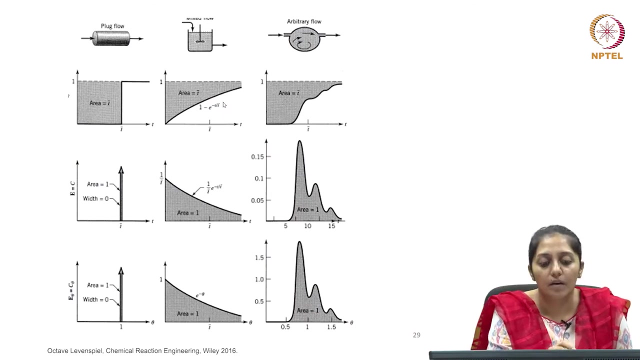 is introduced in the stream of a white fluid being sent in the reactor, the C curve of the tracer. So E becomes equal to C. So if you see on the slide where the first picture shows, a plug flow setup, So the second is your mixed flow and the third is your arbitrary. 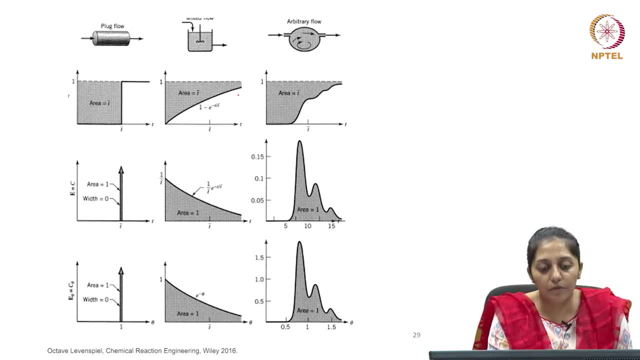 flow. Now for a plug flow. here they have shown a step input. So in case of a step input the exit, if it is a plug flow system, will also be a step change after the release. Now you will just move the gas from an type input, so at f0 to f2.. Now for a plug flow. 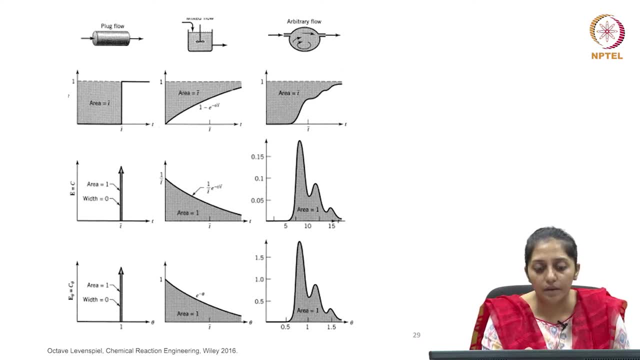 the Harrison test-tv. on the next slide I will show on intensity niemi that больше than seven millones of분. then join like a loop curve with inductance, you will find a full fat бывruster situation. You can see the scale is golden. long with 항, it is golden with touchdown. we can. 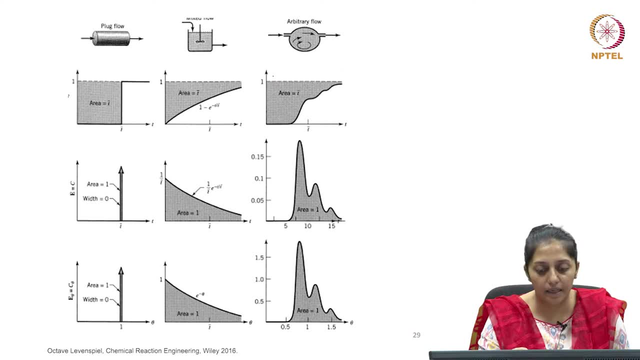 also find wash, and we can perpendicular and trophy. so, Ok, well, now you can see what these small curves are, these curves which gonna to representa that, the anni, so the active force. What else we can see in this line, this display? we can consider what is a thanks for. 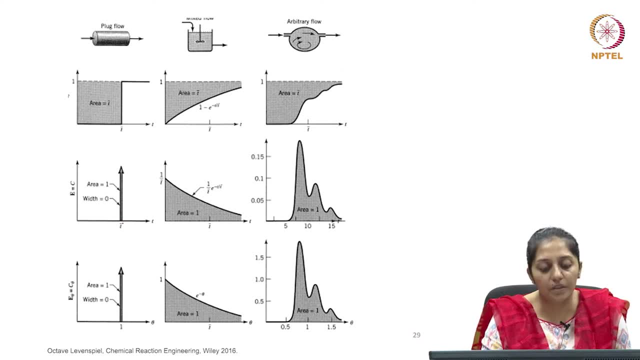 the次 c. then what is the stage? waiting constant from above on f 0 to 1, if it is a check, after the residence time shown here as T bar. Now for a similar impulse, the concentration profile, or where the unit is. so it is a unit impulse. So then E becomes equal to C. 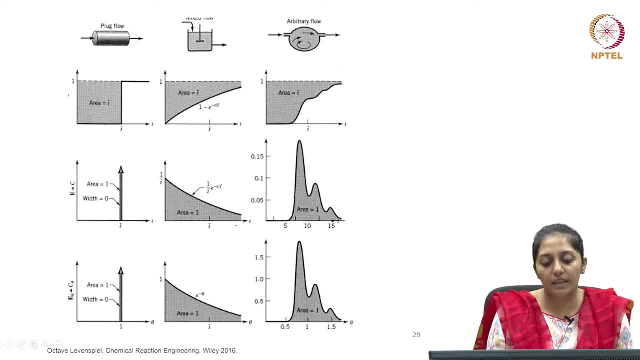 and the exit will be an exponentially decreasing curve. If you convert E in terms of theta, then E theta will also be equal to C theta in case of a unit impulse and similarly, your exponential function will also get converted into the dimensionless form of theta. 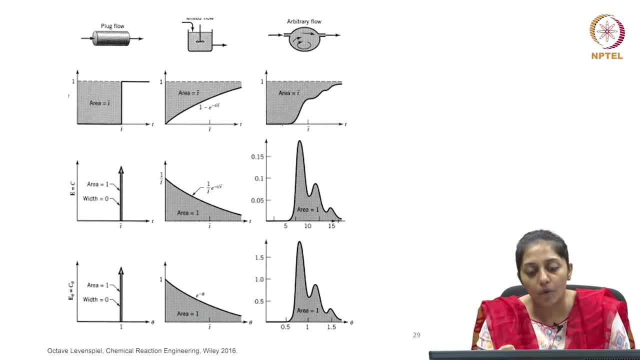 Now, if it is an arbitrary flow, then what you observe may not be an exponential increase, but can be with many peaks. Similarly, for an impulse unit impulse increase, then E theta will also be equal to C theta in case of a unit impulse. 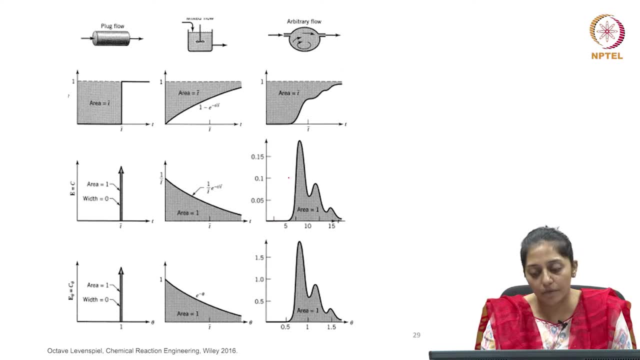 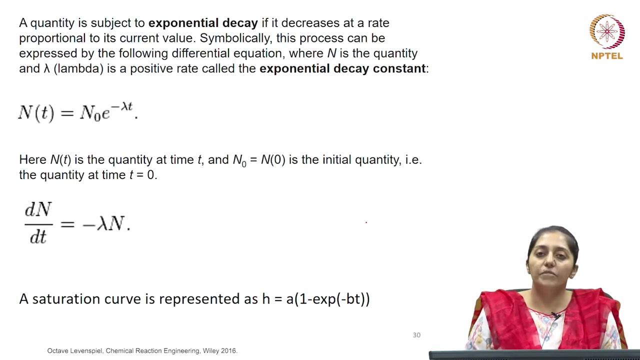 input at the exit for an arbitrary flow, you may observe a lag, as shown in the picture here, and with subsequent, peaks of decreased amplitude can be observed coming out from the reactor, where the total area can be 1.. Now, a quantity is subject to exponential decay if it decreases. 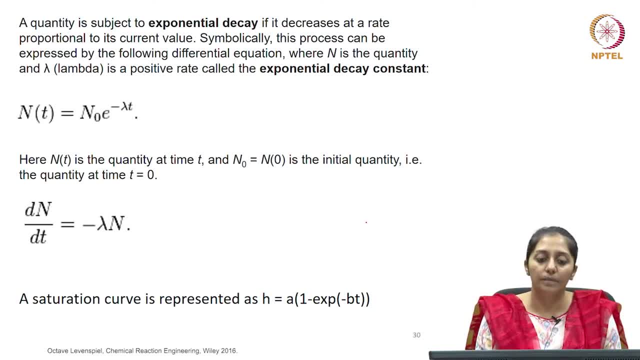 at a rate proportional to its current value. Symbolically, this process can be expressed by the equation shown here. let us call it as equation 1. this differential equation, where the n is the quantity lambda, is the positive rate called as exponential decay constant. Your nt. 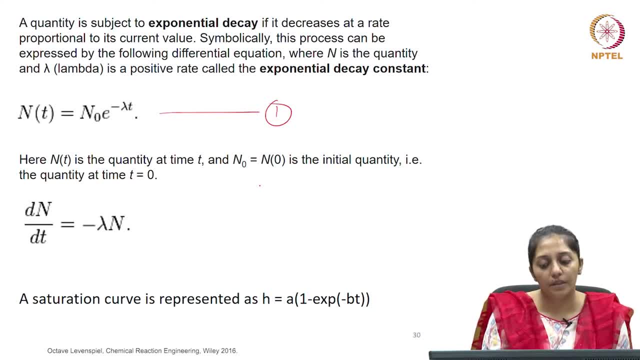 will be the quantity at time t: n0. n0 is the initial quantity, which is at time t. so effectively, the rate at which the n is changing is proportional to n and lambda is your rate constant and because decay. so therefore, the negative sign and a saturation curve will be represented mathematically as shown here. 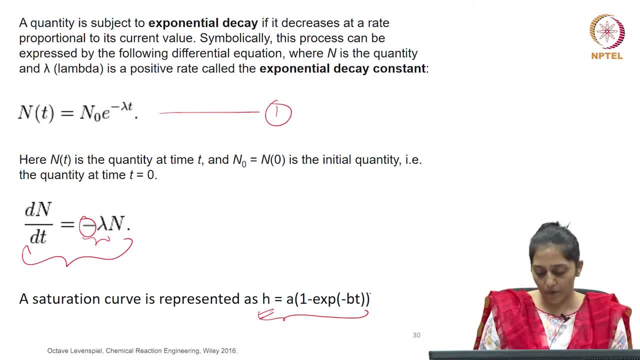 h is equal to a, 1 minus e to the power of t. So the rate at which the n is changing is proportional to n, and lambda is your rate, она minus Batt. so a, b are constants and this is an exponential function with respect. 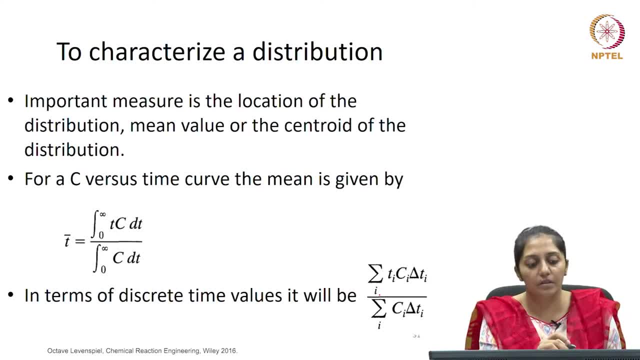 to time. so a saturation curve. now to characterize a distribution. What is important to be measured is the location of the distribution, mean value of the distribution, and the same thing is called as the centroid of the distribution. Similarly, we can generalize the situation with respect to the outcome. Now let us mentioned what I have been simply described here, we can find the different possibilities and types of some of these. Now remember, within the сравdelations are blessings, regardless of on campus var, t, o, z, etc. The Neptunian boundary can be calculated based on balance ofantis, ec, etc. Now do consider our observation, In this case, how the gehelectence器 is marked as Oh, the Schnhaltz universal, and that this or N is the coherent, erroneously being comfortable, yourselves denken along the called these Nson. 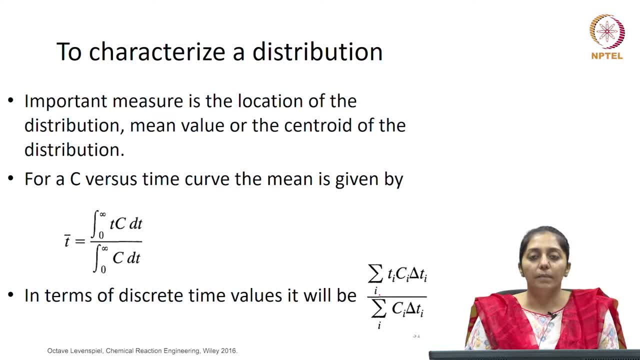 Now for a C versus time curve. the mean can be given as shown here and in terms of discrete time values it can be shown here in the second line. So this is how statistically you can define mean value of time in a C versus T curve. 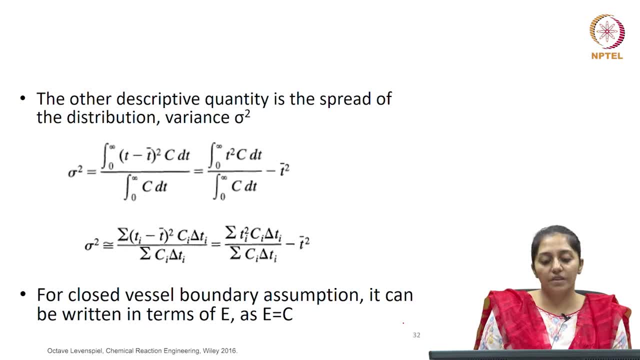 Now the other descriptive quantity is the spread of the distribution, which we call as variance. Now, variance is mathematically represented as the function shown here, let us call it as equation 2- and in discrete time intervals it can be represented as shown in the second. 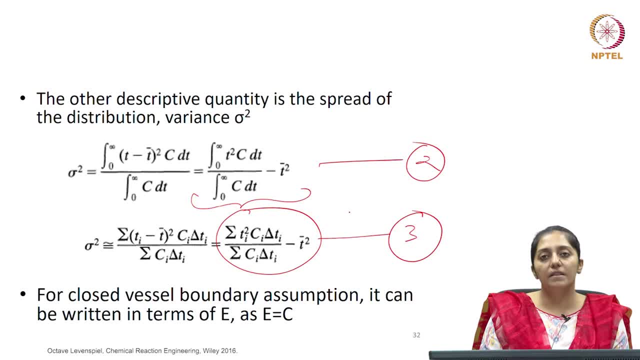 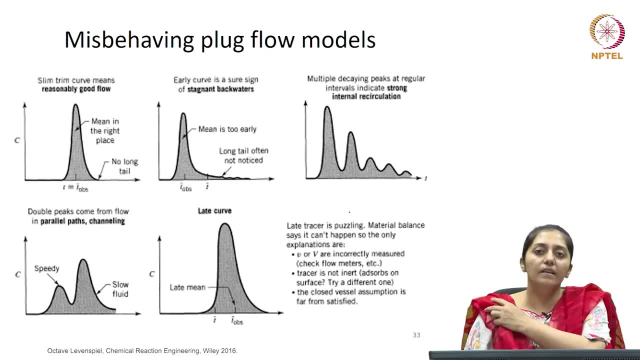 line. Now for closed vessel boundaries. at steady state, your E is equal to C. So how do we practically find out misbehaving plug flow systems or those which are deviating from ideality? Now, if you see at the exit, in a concentration versus time plot, something coming out after, 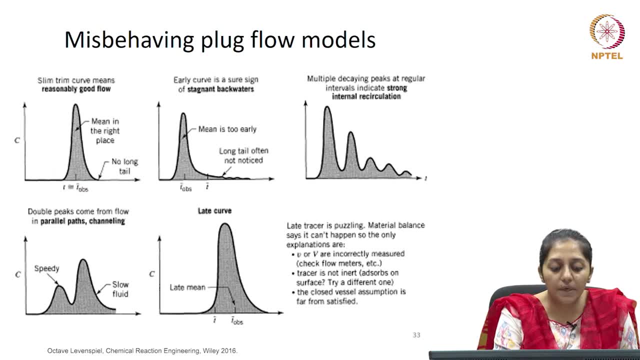 certain amount of time and the mean of the peak which is observed is found to be greater than the theoretical residence time. So this shows reasonably good flow. it is a sharp peak And the mean residence time is equal to T residence time is equal to the theoretical mean residence time, So this T bar is the mean. 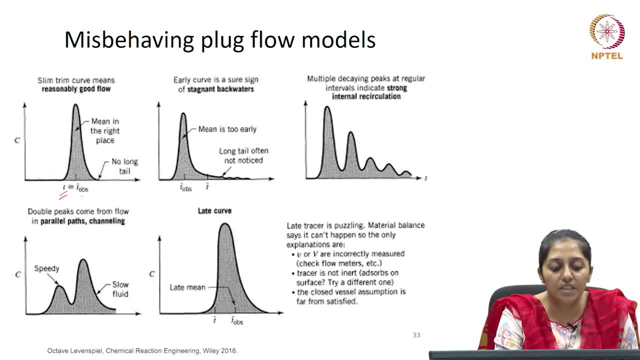 residence time calculated from the C versus T data. T bar observed and T bar would be your theoretical mean residence time. So if both are nearly same and you see a sharp peak in a flow system, coming out with a time mean residence time equal to that of the theoretical residence, 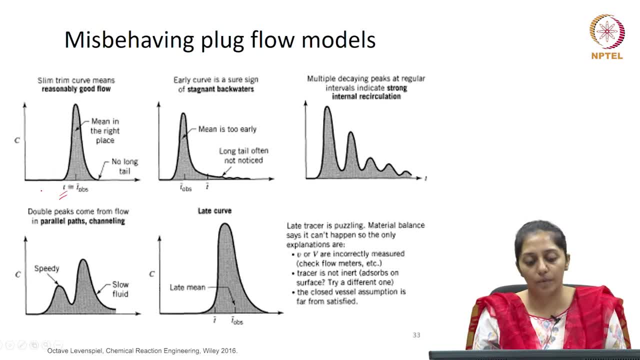 time, then it shows a reasonably good flow. So no long tail. if you see on the picture Now, if there are stagnant backwaters, then your observed mean residence time would come much earlier than the theoretical mean residence time and you will see a long. 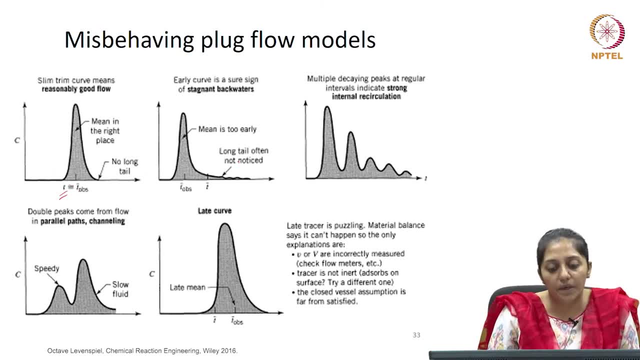 tail at the exit of the material or of the racer. Then in the third scenario, if you see lot many peaks of decreased amplitude, then this shows strong internal recirculation of the medium. This gives an indication of that behavior. Now, if you see only two major peaks, 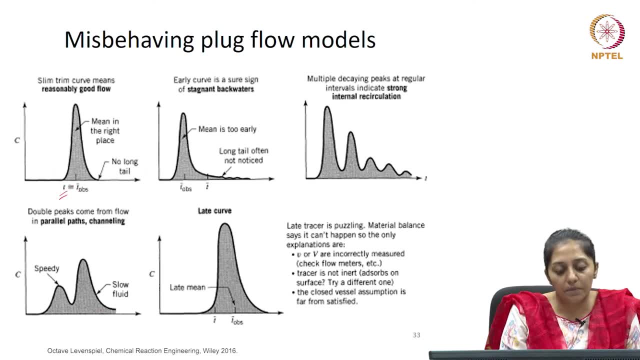 coming at the exit. So the earlier one can be seen as a long tail at the exit of the material can be speedy and the later one can be slow. where your the peak can be, for one is less than the mean residence time. for the other is greater than the mean residence time, So the one can be. 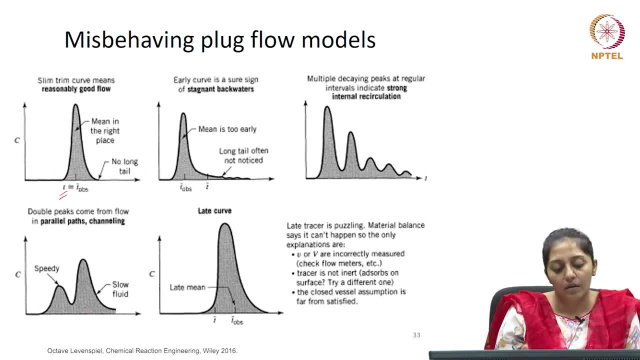 speedy liquid flow and the other fluid elements can demonstrate slow fluid movement. So this indicates parallel paths inside the reactor or channeling. Now, if you observe a very late curve exit of the material tracer from the reactor with the mean residence time observed being greater than 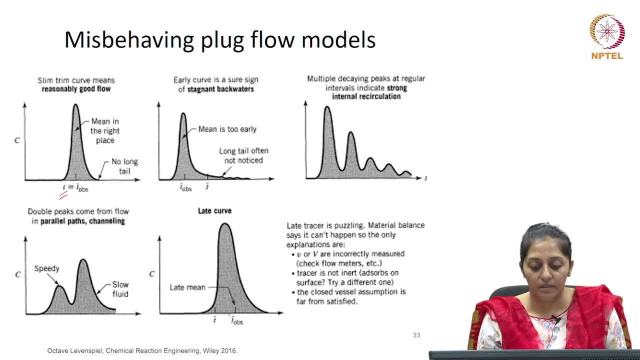 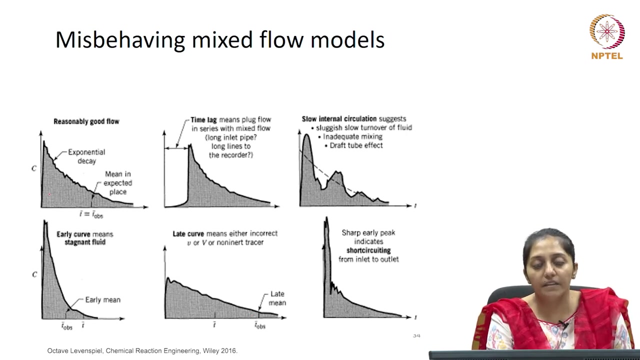 the theoretical residence time, then this indicates either the volumetric flow rate or the volume have not been measured properly, or the tracer may not be inert, might be getting absorbed, or the closed vessel boundary Assumption is not getting satisfied. Similarly for mixed flow models: how to find deviation? 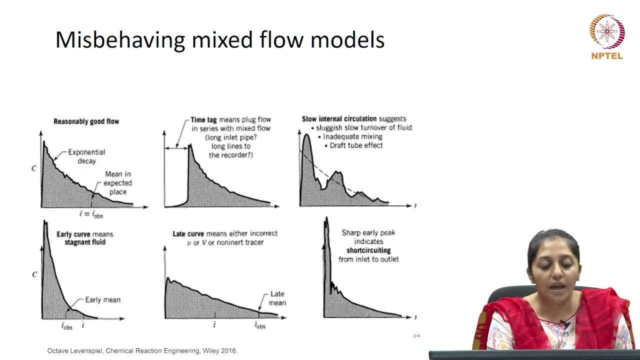 from ideality Now for an ideal or reasonably good flow. in a mixed flow model for a pulse input, the concentration of the tracer will show an exponential decay and your mean residence time. Now, if you observe a very late curve exit of the material tracer from the reactor or channeling, 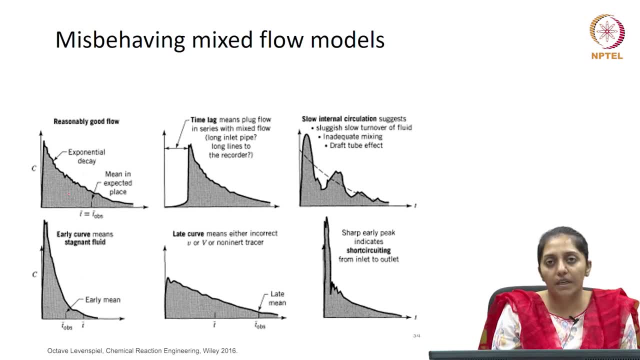 then this indicates either the volumetric flow rate or the volume have not been measured properly or theйne residence time observed would be equal to the theoretical residence time of the reactor. Now, if you observe that there is a lag and then you observe a sudden rise in the concentration, 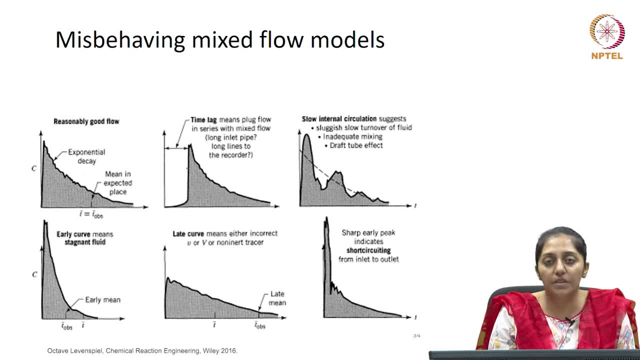 with subsequent exponential decay in the C versus T curve, then this would mean that either there is a very long inlet pipe, which indicates long lines for recording. So either at the exit or at the entry there are long pipes, So there is a lag due. 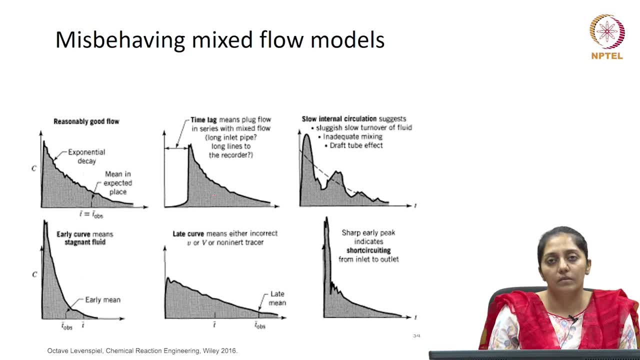 to this path covered by the fluid elements at the exit or at the entry. Then if you observed peaks, more than one peaks, coming out at some intervals with decreased intensity, then this would mean inadequate mixing or maybe the draft tube effect, the internal recirculation. 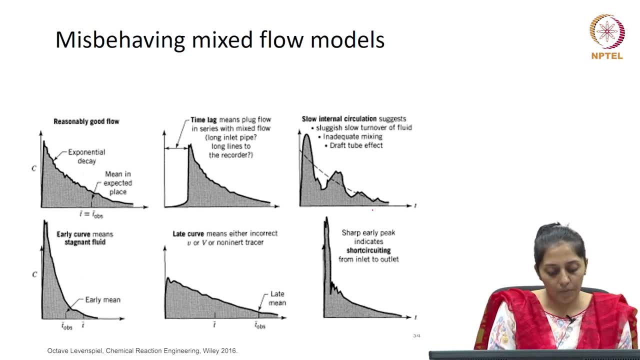 If your mean residence time observed is found to be early than the theoretical mean residence time, this would mean stagnant zones in the reactor because of which the path being covered effectively has been reduced. So most of the liquid individual stickiness is low, So this means that you could have a higher rises than in the todays objective method, as we could have seen in the previous thoughts. 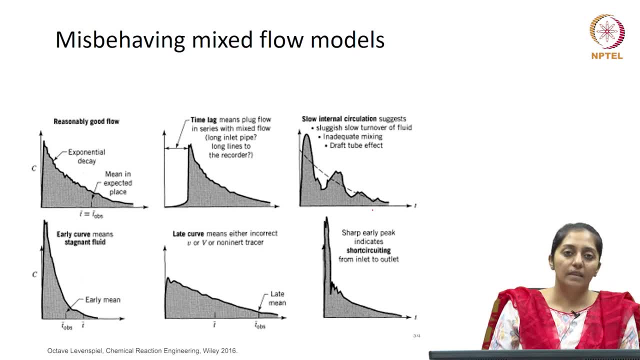 So that means if you observed peaks, more than one peaks coming out at some intervals with decreased intensity, particles are spending less time than the theoretical residence time. Now, on the contrary, if there is a late curve, which means your mean residence time observed is found to be later, 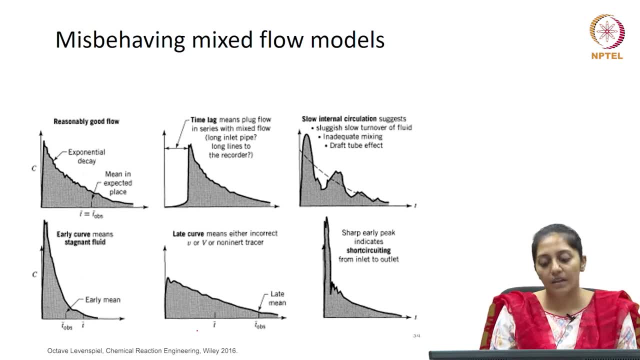 much later than the theoretical residence time. this would indicate either incorrect measurement of the volumetric flow rate or the volume of the reactor, or the tracer is not inert Now very sharp early peak. this might indicate short circuiting from inlet to the outlet and then suddenly it dies down. So this can be due to the result of 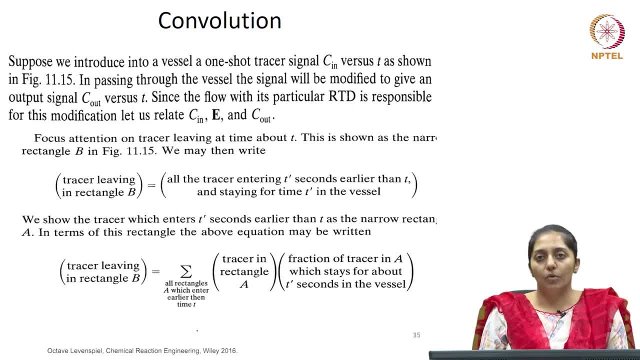 short circuiting. Now, whatever we have been spoken or we have derived up till now has been for a non-reactive system. Now, how can we relate the residence time distribution or this non-ideality? how will it impact the reaction or the performance of the reactor? Let us see and characterize. 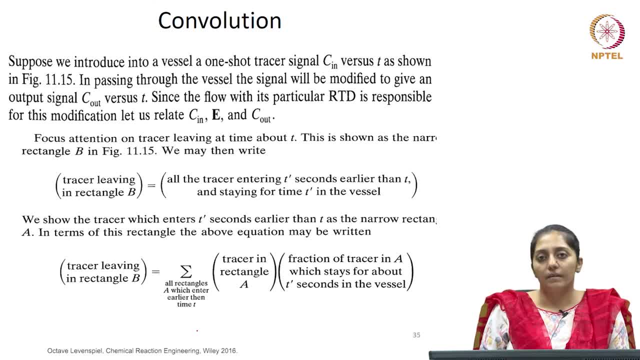 that Now, in order to characterize that, we need to determine the non-reactive system. Now, in order to determine the non-reactive system, we need to determine how the concentration at the inlet and the concentration at the outlet are related to the mean residence time distribution, So that in case of a non-ideality. 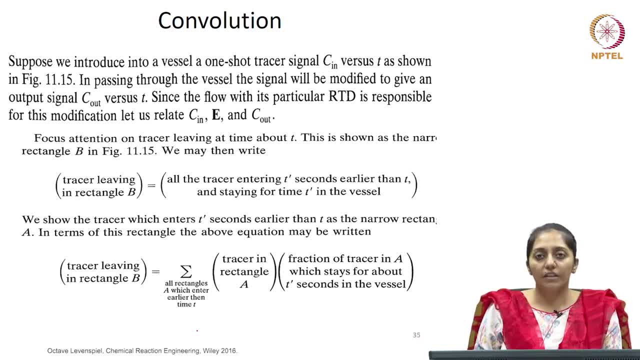 one can take into account what will be the actual reaction, kinetics and the performance. So in order to derive that, let us first see how C in and C out are related to the mean residence time distribution. So in order to derive that, let us first see how C in and 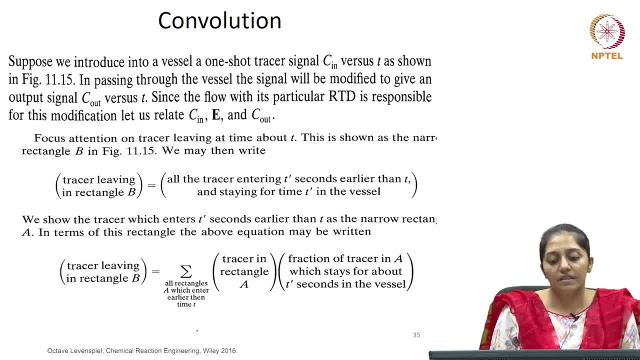 C out can be related with the residence time distribution or the E value. Now suppose we introduce in a vessel one shot tracer, let the signal be C in, and this tracer is not a pulse tracer but it is an entire profile of C in versus T. so this is a curve signal. 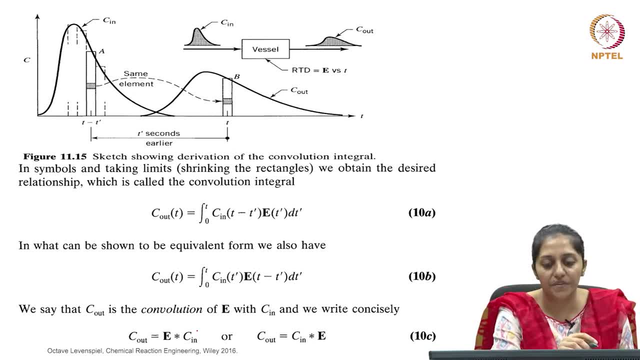 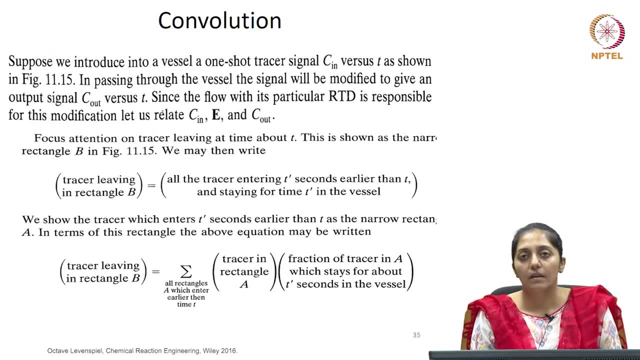 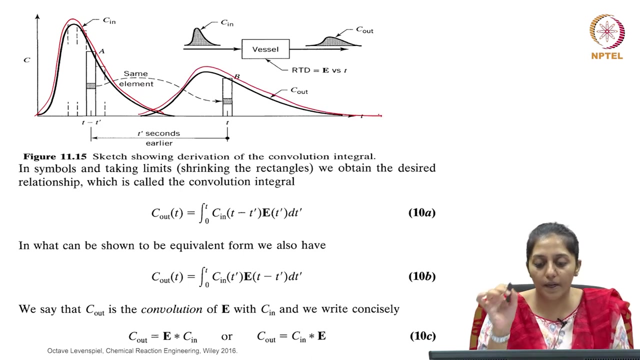 Now you can see it on the slide here. So this portion is your C in. Now, while passing through the vessel this signal may get modified to get the C out signal. So let us assume we were able to see this profile at the exit Now, since the flow with its particular residence time distribution. 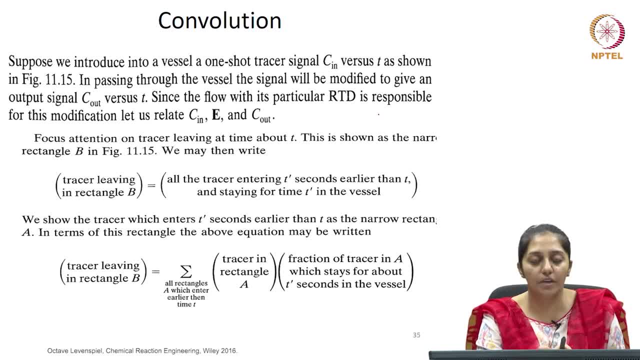 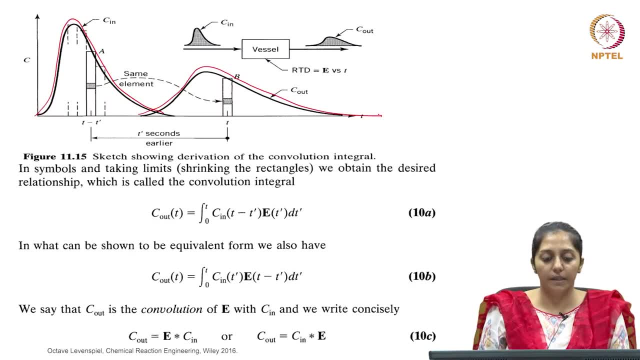 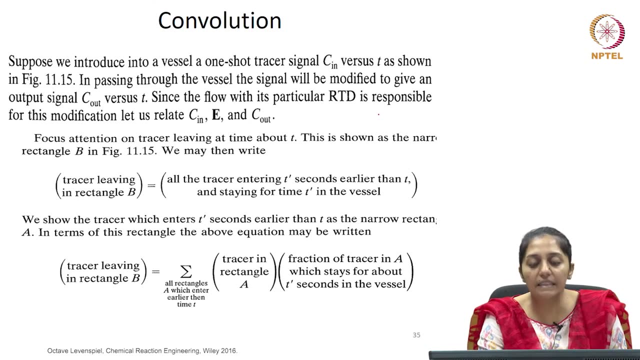 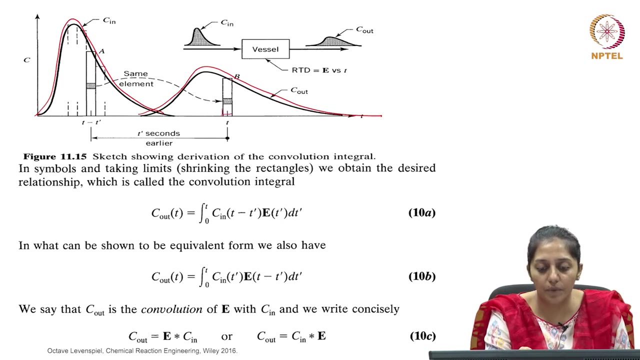 is what is responsible for this modification of the curve of C in and C out. let us try to connect it with the RTD. Now focus your attention on the tracer which is leaving at time T So, which is shown here. So this is the fluid element marked as B which is leaving the reactor at time. 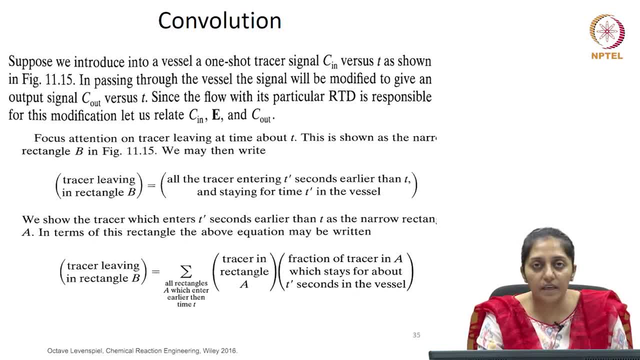 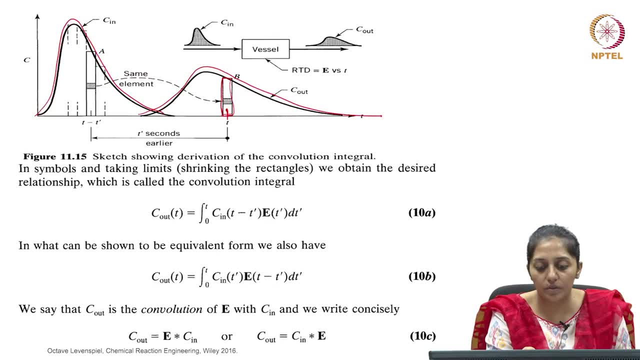 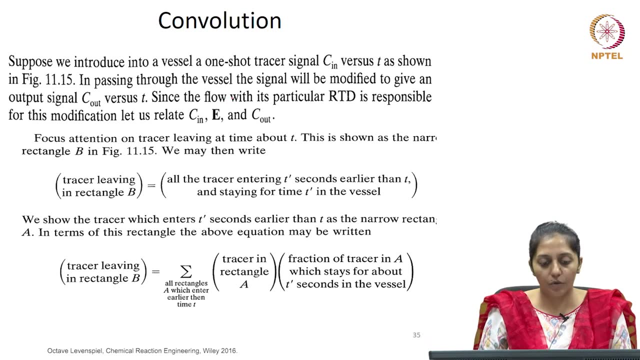 T, So this is the fluid element marked as B which is leaving the reactor at time. T, So the tracer in this rectangle B will be equal to. so let us see this: So grape box, So the amount of tracer in this rectangle B. how do we determine? So the tracer which is 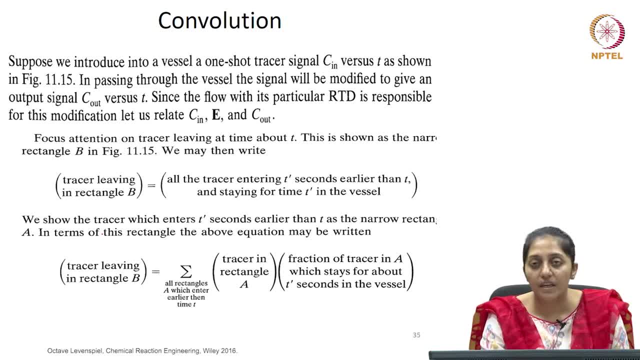 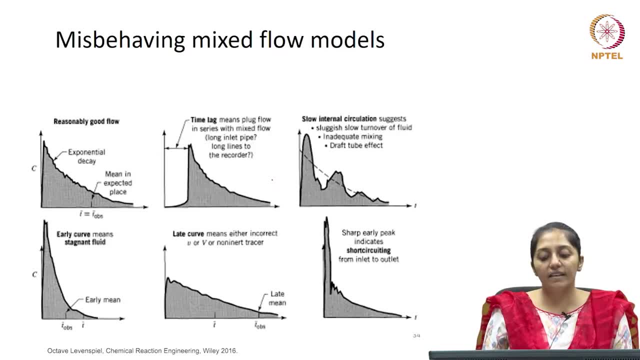 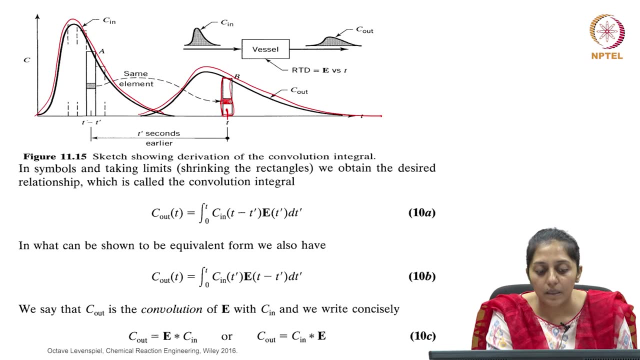 leaving in this rectangle, B fluid element is nothing but all the tracer entering at T prime seconds Earlier than T. Now, what was T prime? T prime is nothing but the corresponding element. It is the same fluid element which is in the inlet now being called as A. 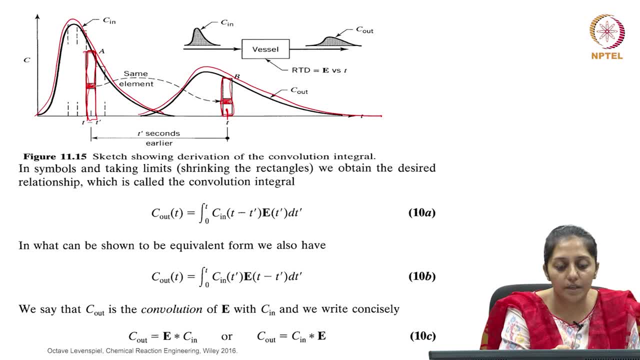 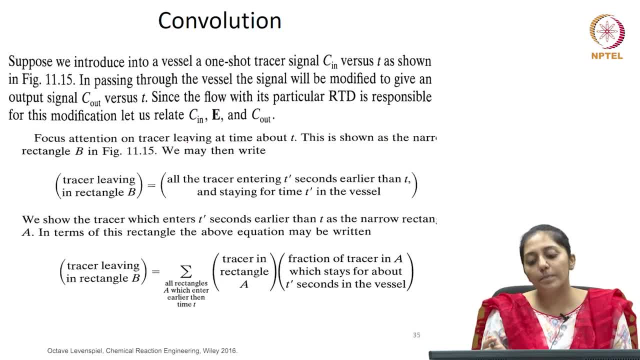 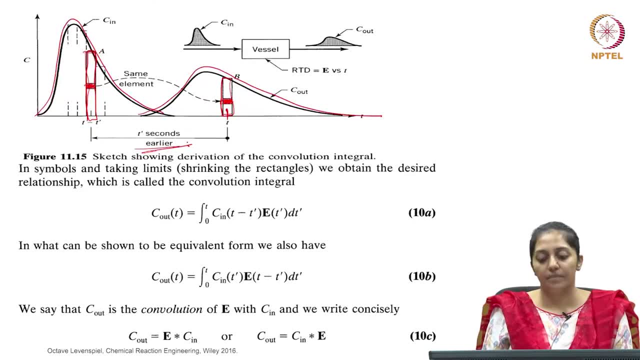 All the tracer entering T prime seconds earlier than T and staying for T prime in the vessel. So whatever tracer we measure here at time, T is nothing but all the tracer which must have entered the reactor before T prime seconds and which must have stayed in the reactor for T prime seconds. Now we show that the tracer 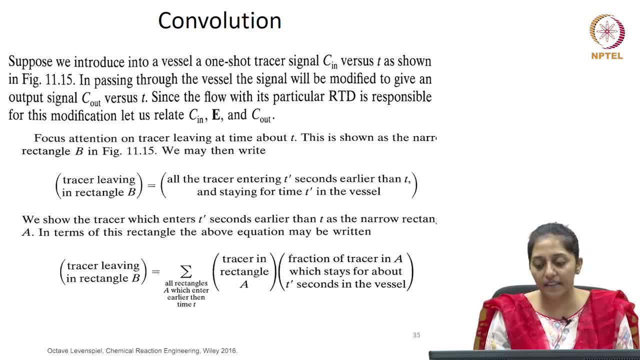 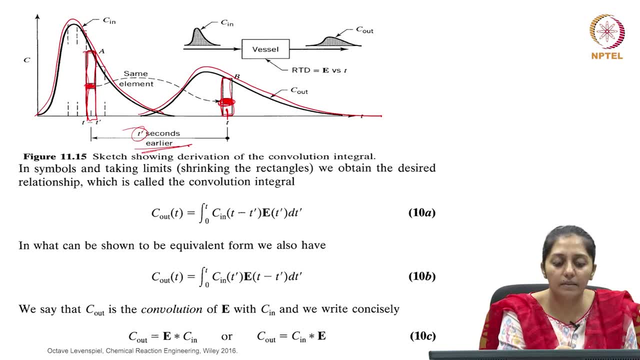 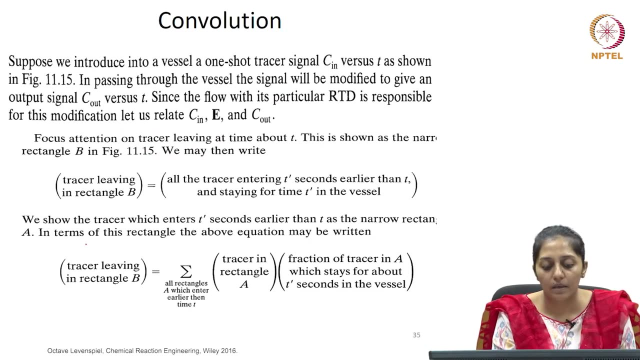 which enters T prime seconds earlier than T as a narrow rectangle A. This was the same element at the before T prime seconds. Now, in terms of this rectangle, the above correlation can then be written as: let us see: tracer leaving in rectangle B is equal to summation of all the 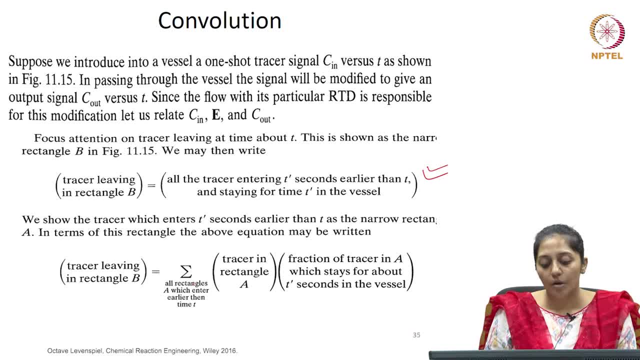 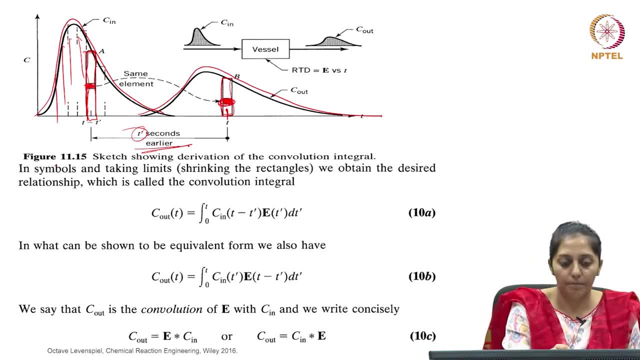 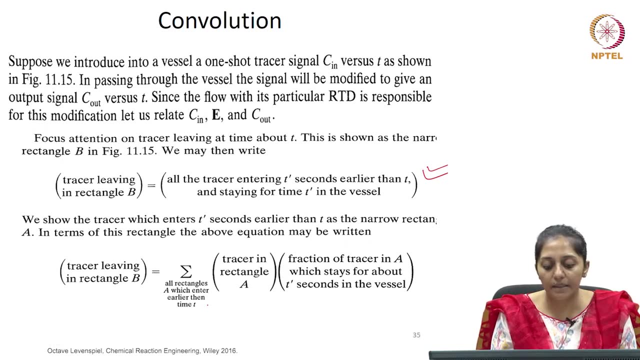 rectangles A which have entered earlier than time T, So which means similar such all rectangles Before time T. Now, in terms, all the rectangle A's which enter earlier than time T, the summation of all such rectangles having what the tracer in all these rectangles, multiplied by the fraction, 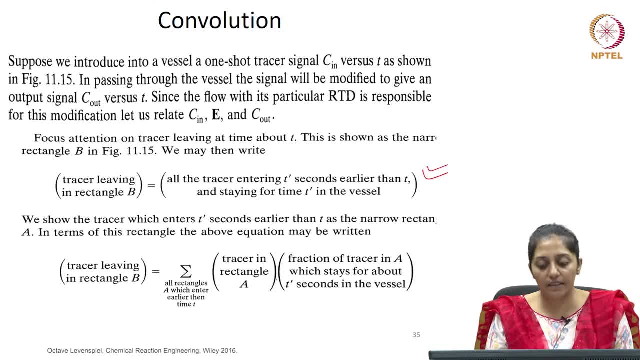 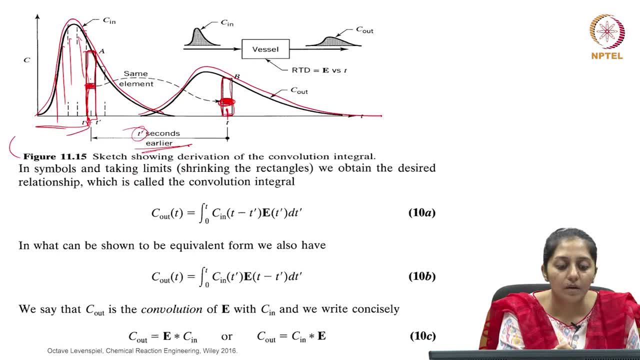 of the tracer in each of these rectangles which stays for about T prime seconds. So not all the tracer here is spending only T prime seconds in the reactor. So among all these rectangles, the fluid elements, we need to find the fraction of those tracers which have spent. 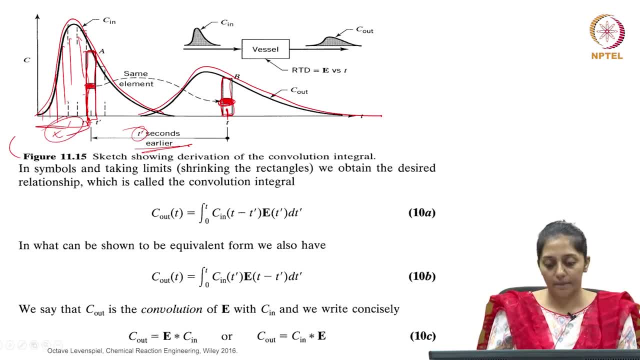 T prime second inside the reactor. So this means what? that the concentration at the output at time. T is the concentration of the fluid elements before T prime entering the vessel. residence time distribution: This is nothing but E. T prime is the fraction of the tracer. 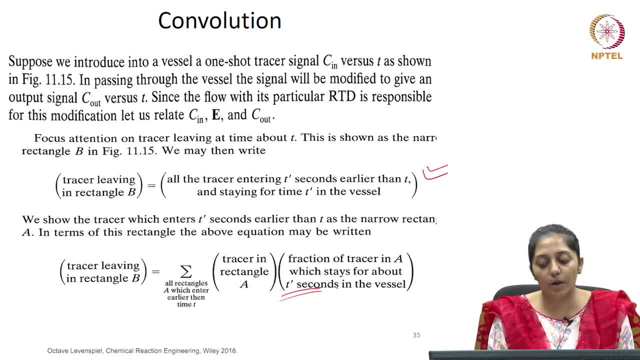 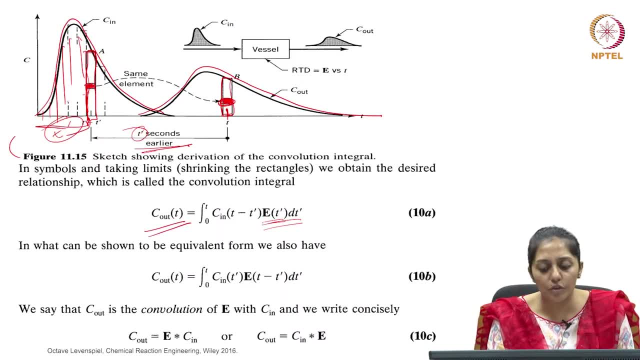 in the fluid element which stays for about T prime seconds in the vessel. So this is nothing but E T prime as per the definition of the E curve. So the fraction of the fluid element which is staying for about T prime seconds in the vessel. So this is nothing but E T prime. 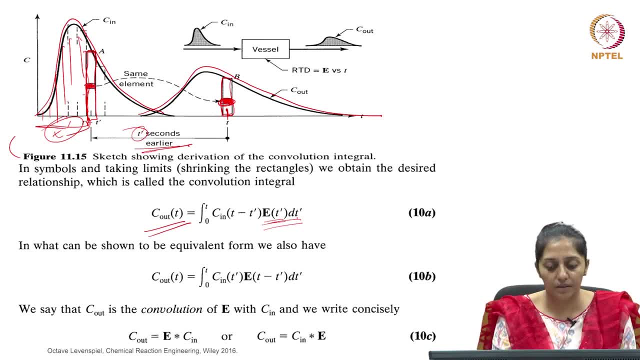 the time t prime. This is et prime dt Now. here the integral will be all those elements up till the time t. So the limit for integration would be 0 to t. So we need to consider all the elements which have been entering and before time t. Now, with the law of convolution, 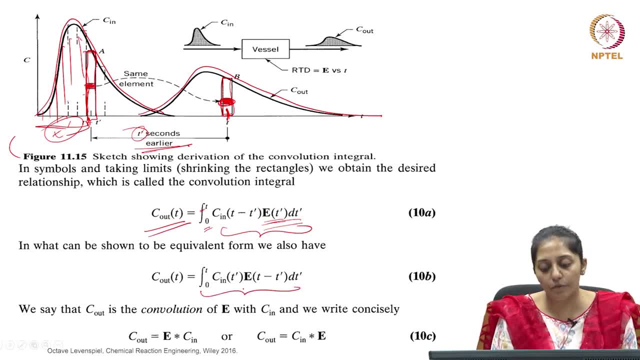 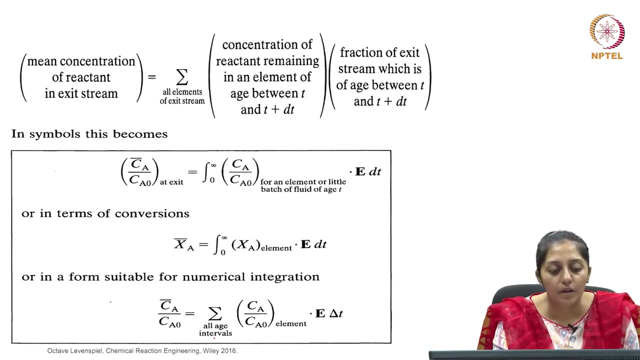 this integral can be rewritten in the form of 0 to t c in t prime et minus t prime, dt prime. So your c out becomes nothing but the exit edge distance Distribution multiplied by c in. Now let us say it is reacting, So mean concentration of the. 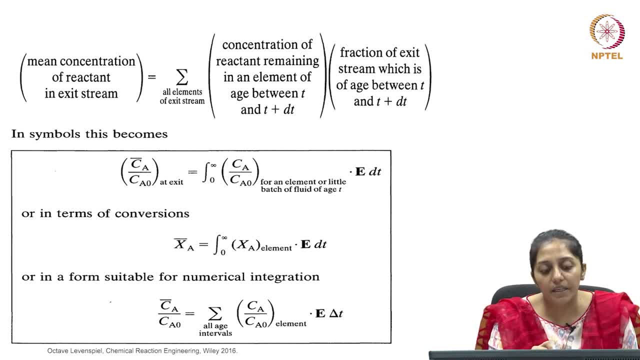 reactant in the exit stream will be equal to all the elements of the exit stream and the summation of all such elements and summation of what: The concentration of the reactant leaving in an element of age between t and t plus dt And the fraction of the exit stream which is of age between t and t plus dt. So first we need to 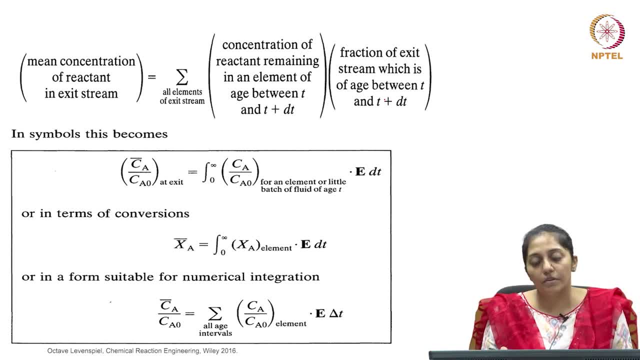 find out the fraction of those exit stream which are of the age between t and t plus dt and multiply it with the concentration of the reactant remaining in any element between the age t plus t, dt, t and t plus dt. So now, in terms of the concentration of the reactant, 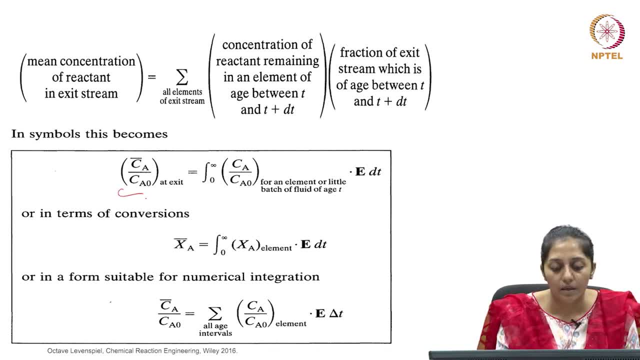 we can define the convergence of symbols and the mathematical form c a prime by c a naught. So this is at the exit fraction of conversion. So this becomes your conversion, which is called as x a. It is 0 to infinity, all the elements of the exit stream. So we are having the limits as